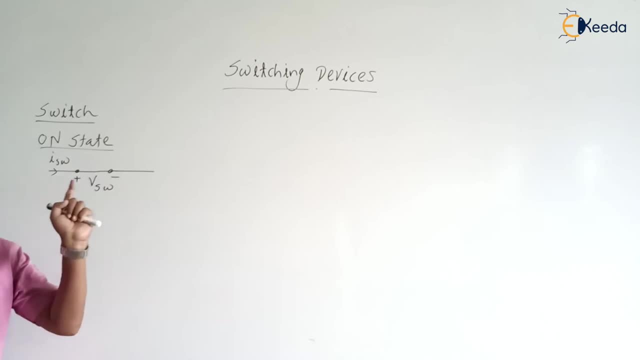 So VSW is the voltage across the switch, ISW is the current flowing through the switch. okay, Next, similar to the on state, we are having one more state, that is, the off state. Off state: The switch is said to be in the off state. The switch is said to be in the off state. 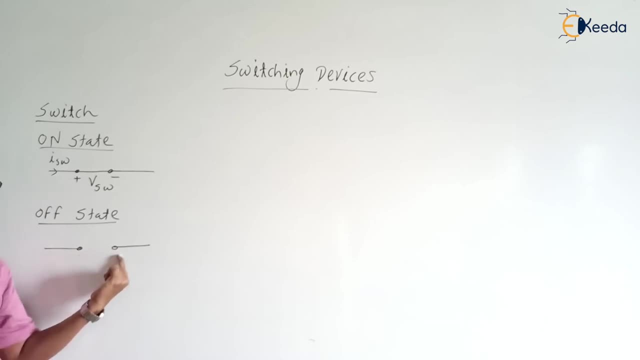 If there exists a closed path between these two terminals, then we generally say that the switch is on. If there exists the on state, the switch is on. It can be said that the switch is closed and the terminal is in the off state and the terminal is closed. 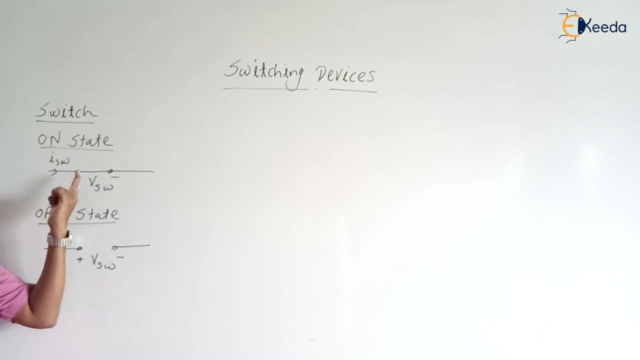 So that is the closed path between these two terminals. okay, Here it is a VSW, there is a ISW. okay, So we are having the on state of the switch and the off state of the switch. If there exists a closed path between these two terminals of the switch, then we can say that the switch is in the on state. 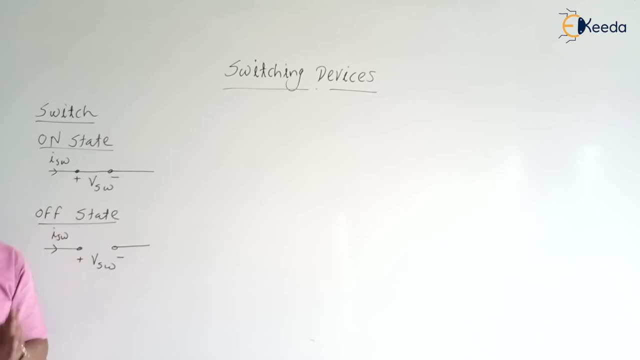 in the open circuit or switch is in the off state, okay now. so now, apart from these two, we are having one more term, that is, a power loss. power loss in switch: okay, power loss in switch. as we know, the power in electrical circuit, or the in electrical engineering power is equal to product of voltage. 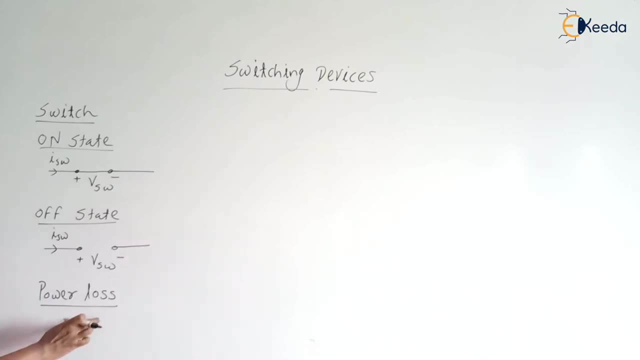 and current right. so here, if we want to find the power loss in the switch- okay, so can we write it as psw- is equal to what power loss in the switch when switch is in the on state, as well as the power loss in the switch when switch is in the off state? okay, so it is like a addition of this. 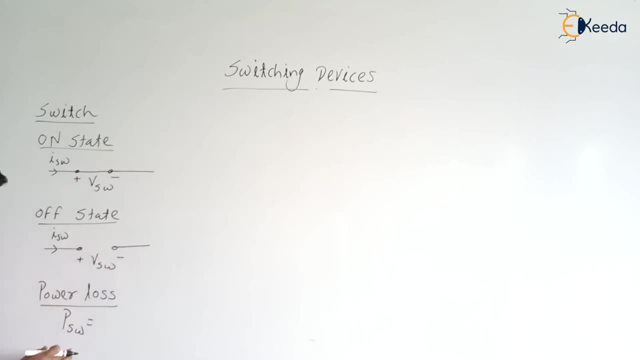 power loss plus addition of this power loss. so can we write it as psw is equal to vsw into isw when switch is in the on state, plus, yes, switch voltage into switch current when switch is in the off state. right, so here total power loss of the switch is equal to what the power loss when the switch is in. 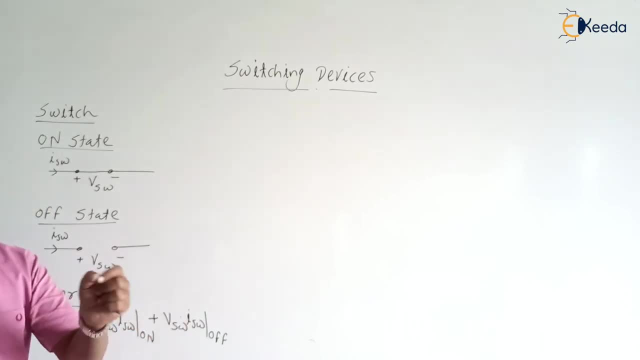 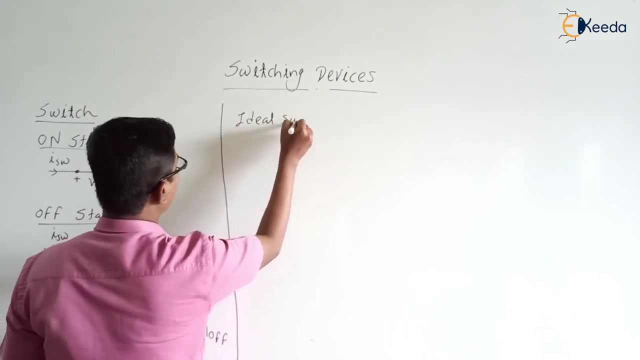 the on state plus the power loss when the switch is in the off state. are you getting the point? okay, so this is about the switch. now we are going to discuss what is the ideal switch and what is the practical switch. okay, so next, ideal switch. ideal switch, okay, ideal switch. so when? an ideal switch? 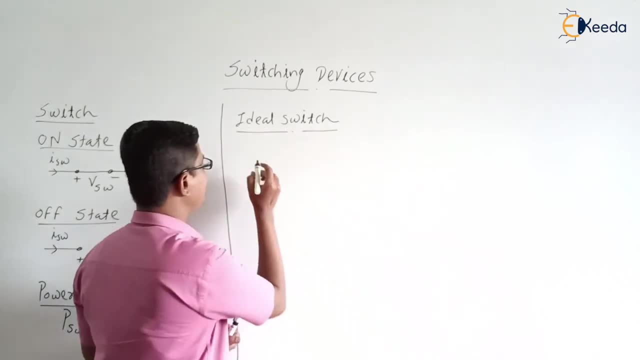 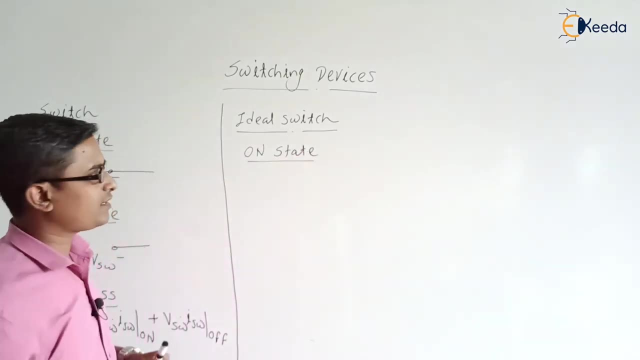 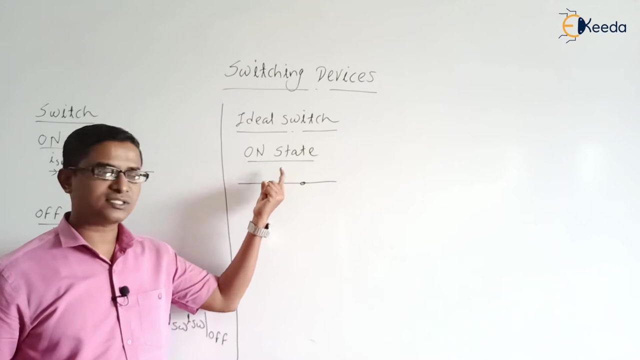 is in the on state. when the ideal switch is in the on state. okay, so ideal switch is in the on state. yes, at that time the switch will behave as a perfect short circuit. the switch ideal switch when is it is in the on state, it behaves as a perfect short circuit, right? so this is the voltage. 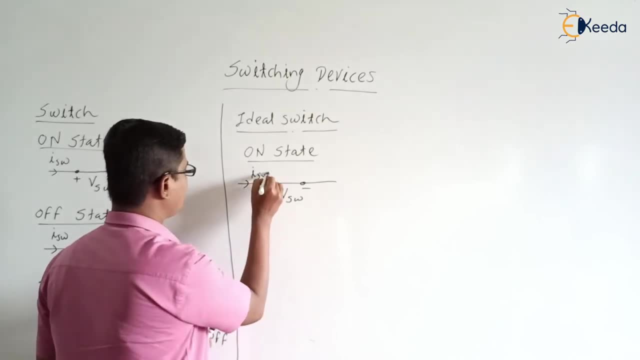 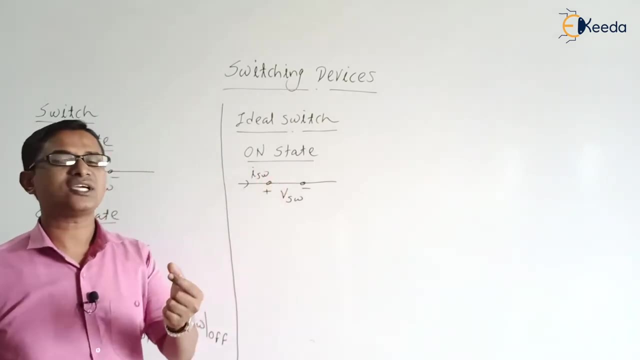 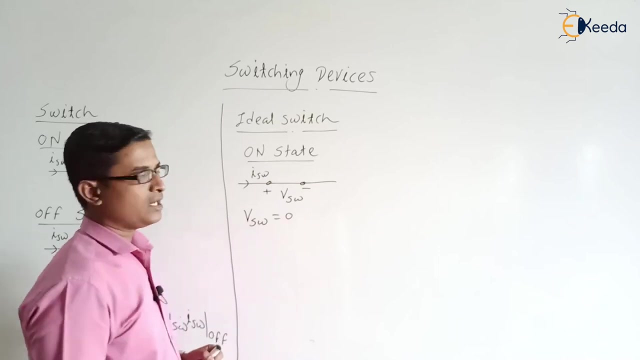 across the switch. vsw. this is the current flowing through the switch. that is a isw, okay. so here as the now we get an ideal switch. if i can divide as one right, which is the current flowing through the switch. this: okay, this is being applied against the speed of this switch. okay, this means that 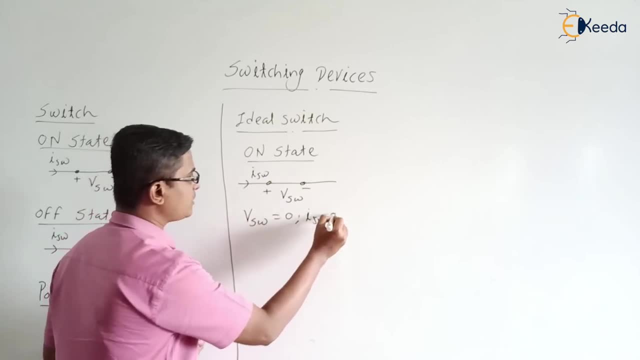 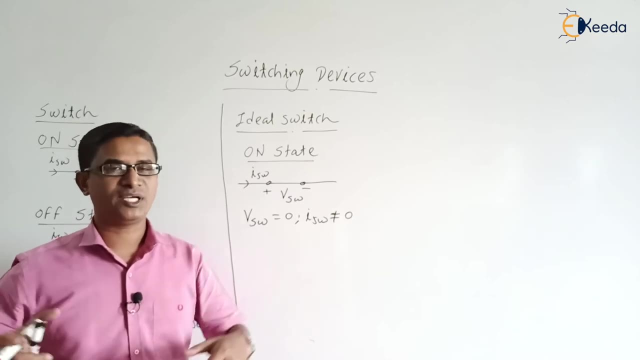 i will be. voltage graph being applied against the speed of this switch. that is totally different. so this is the current flow Senowal and this is the ticket of the short circuit. that should not deviate from the short circuit when i say this is a perfect short circuit, okay, what is the voltage? 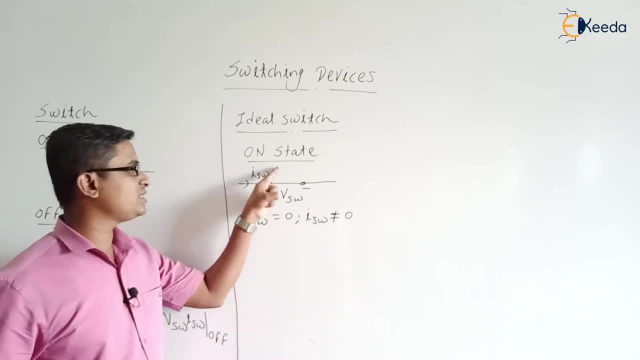 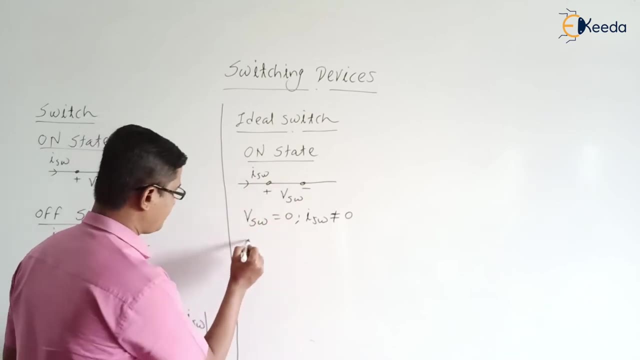 across the perfect short circuit branch. it is a particular right, so can we write it as a vesw equals across. the switch is zero. when current flowing through the switch is non-zero: okay. next, when ideal switch is in the off state. when ideal switch is in the off state, okay. ideal switch is in the 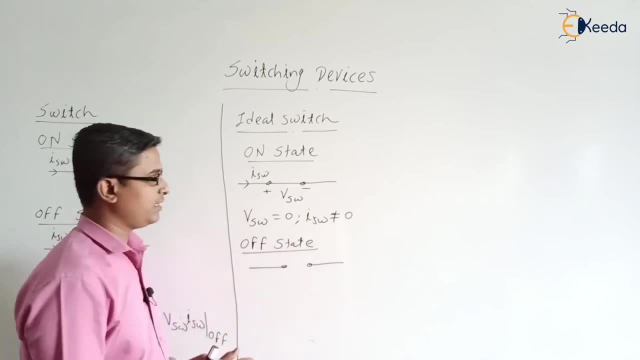 off state means it is acting as a perfect open circuit. it is acting as a perfect open circuit, so this is a vsw voltage across the switch: isw current flowing through the switch. okay now, as this switch is acting as a perfect open circuit, as we know, in the case of perfect open circuit, 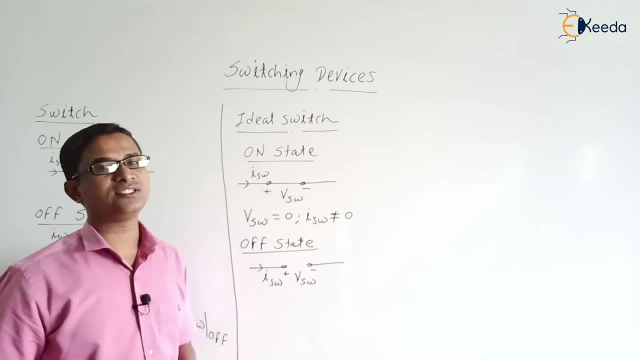 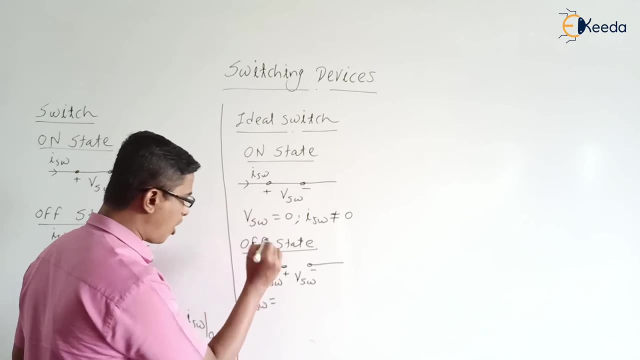 what is the current flowing through the circuit? current flowing through the circuit is zero. okay, so here can we write: in the case of open circuit or in the case of ideal switch, when it is in the off state at that time, what is the current flowing through the switch? it is a zero ampere. 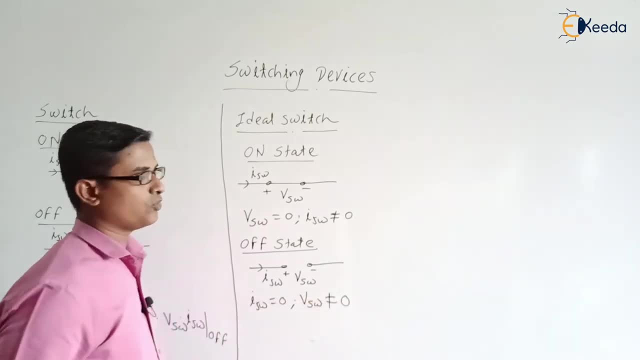 and what is the voltage across the switch? it is a non-zero volt. are you getting the point? okay? so when ideal switch is in the on state, the voltage across the switch is zero, current is acting as a perfect open circuit, as we know, in the case of perfect open circuit, 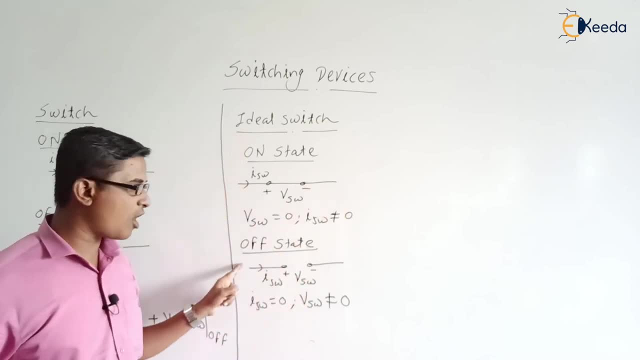 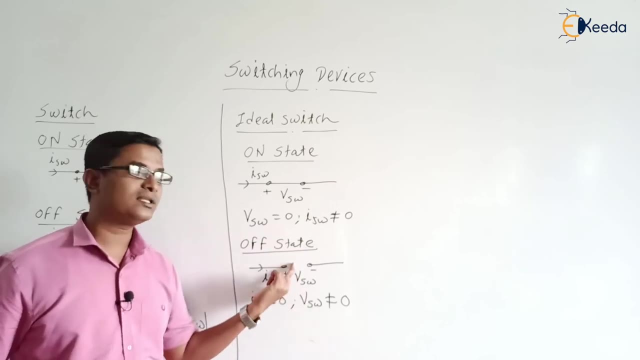 current flowing through the switch is non-zero. When ideal switch is in the off state, the current flowing through the switch is zero, but voltage across the switch is non-zero And important to note- here the ideal switch is acting as a perfect open circuit. Here the ideal switch is acting as: 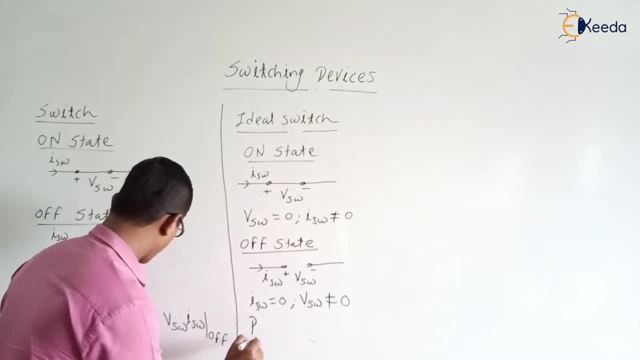 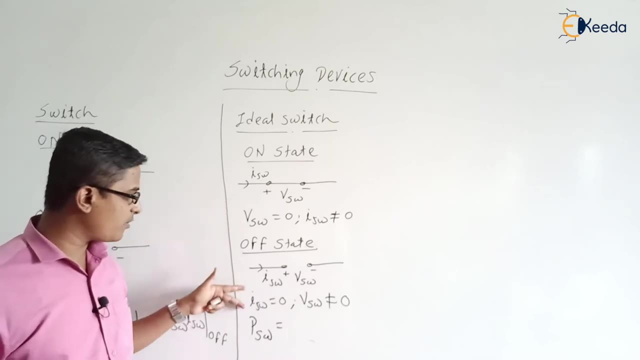 a perfect short circuit. okay. So what is the power loss? in the case of ideal switch, that is, a PSW, It is like power loss when switch is in the on state plus power loss when switch is in the off state. okay, So when switch is in the on state, what is the power loss? It is a zero into. 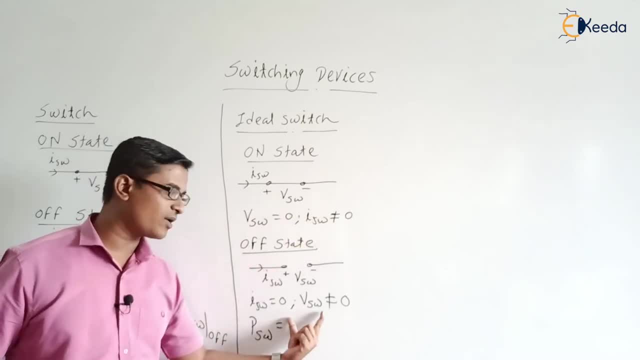 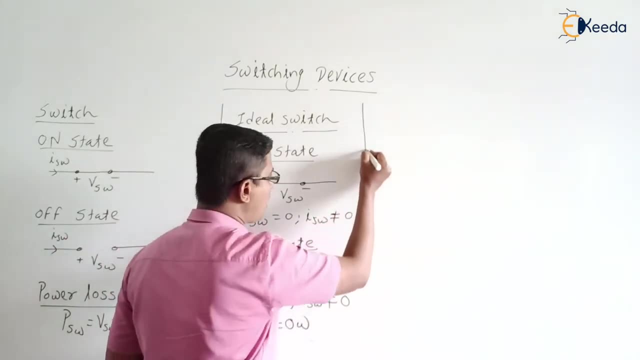 non-zero. So it is a zero. When switch is in the off state, what is the power loss? It is a zero into non-zero. So again it is a zero. So here can we write: when ideal switch is in the on state. 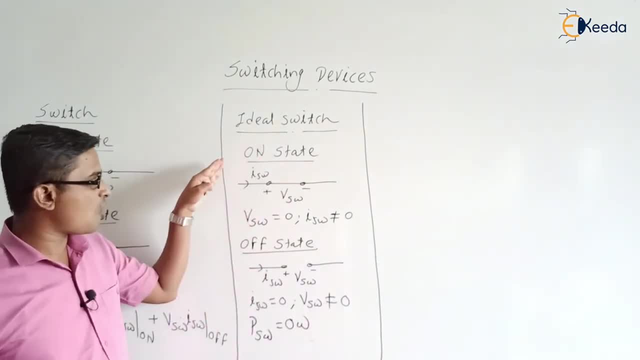 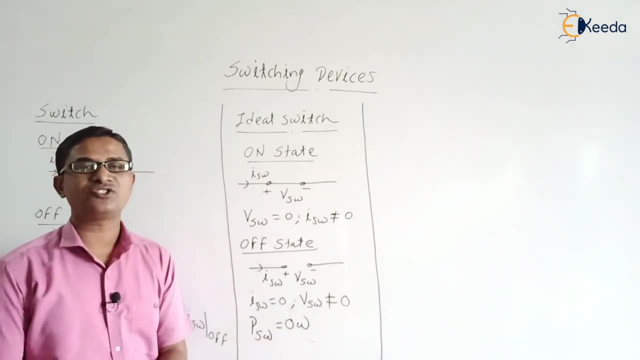 when ideal switch is in the on state, power loss is zero. Ideal switch is in the off state, then also the power loss is zero. So what is the total power loss in the case of ideal switch? It is a zero only. okay, Now, moving towards the next. 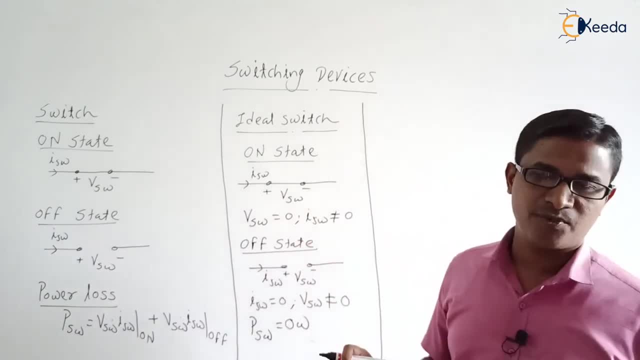 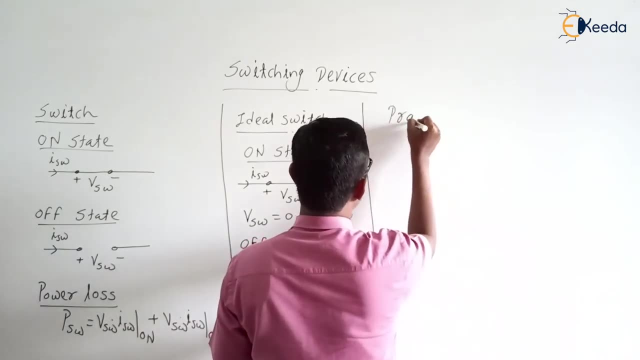 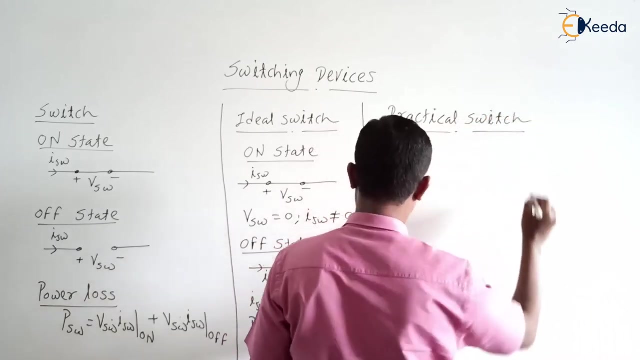 As we know, the ideal things does not exist in real life. okay, So in real life, we are having the practical switches. okay, So let us discuss about the practical switch. Practical switch, Practical switch. right. So now in the case of practical switch, 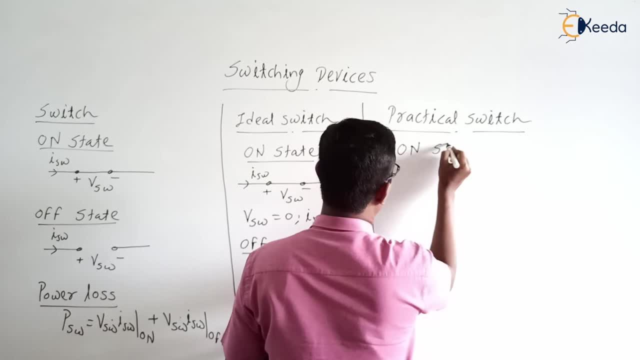 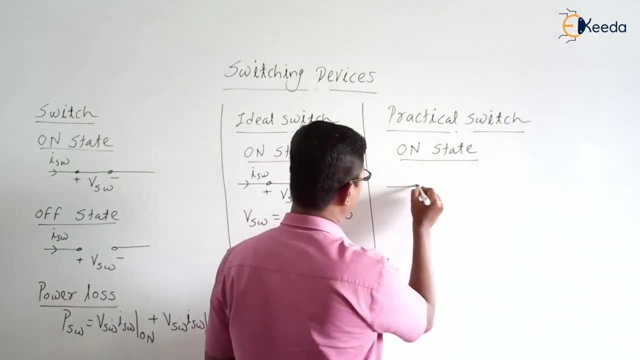 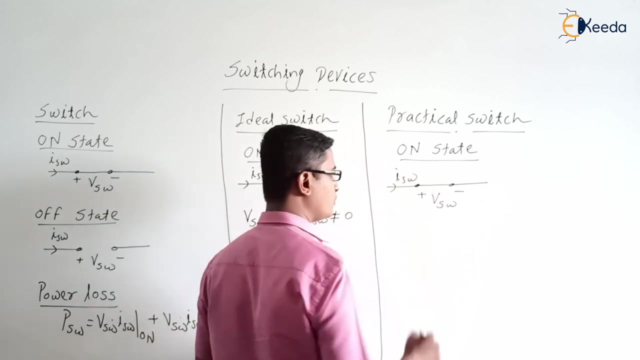 when practical switch is in the on state, then what will happen? Yes, switch is in the on state means it is acting as a closed switch right. So here it is. a voltage is VSW, current is ISW. 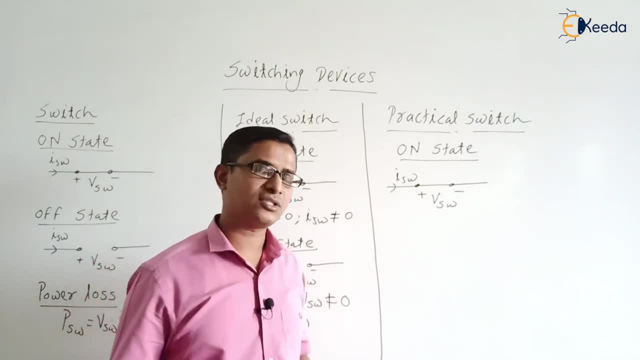 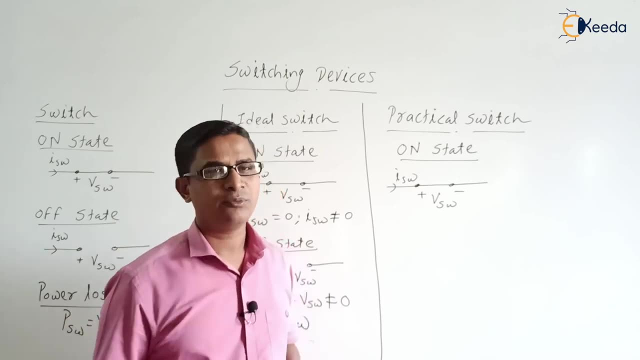 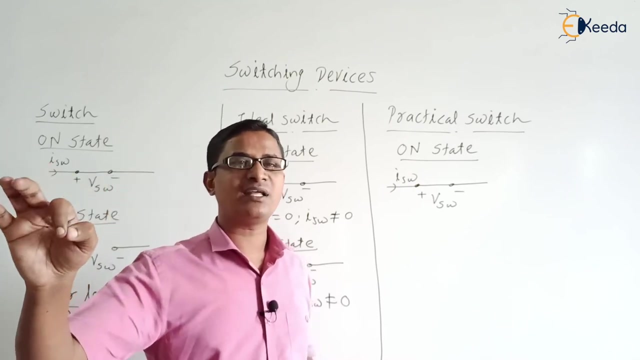 okay, But, as I said, the ideal thing does not exist in real life, okay. So we are having the switch and definitely for that switch, we have used some material right And that material is having some resistivity right And that resistivity of the material is non-zero. So, due to that, what will? 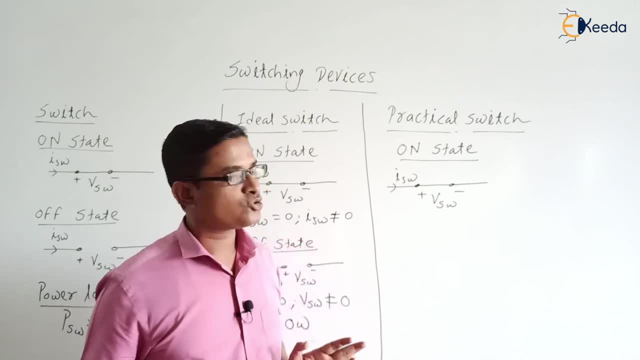 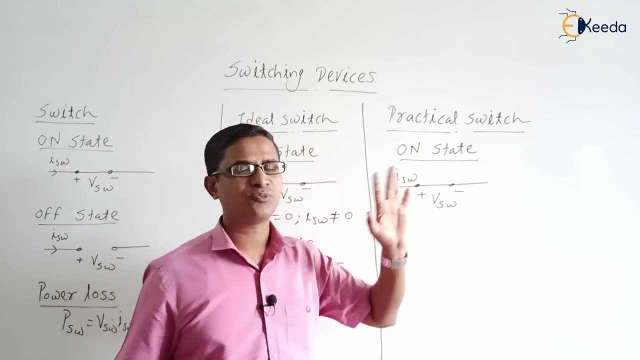 happen, We will be having some equivalent resistance, right. So here, if we replace these two points of the switch with the equivalent resistance, okay, Some small resistance okay. And when the some current flows through that equivalent resistance according to the Ohm's law, what is? 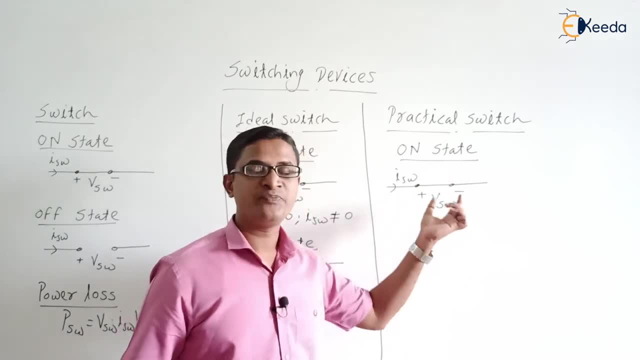 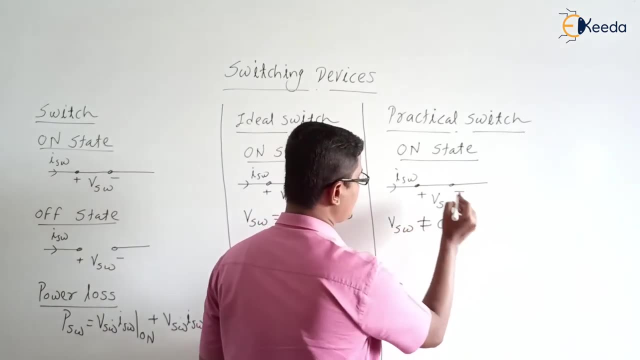 the voltage across that resistance. That is nothing but the voltage across the switch. That is nothing but the VSW. okay, So here we can write it as VSW will be non-zero. Also, what is ISW? ISW also. 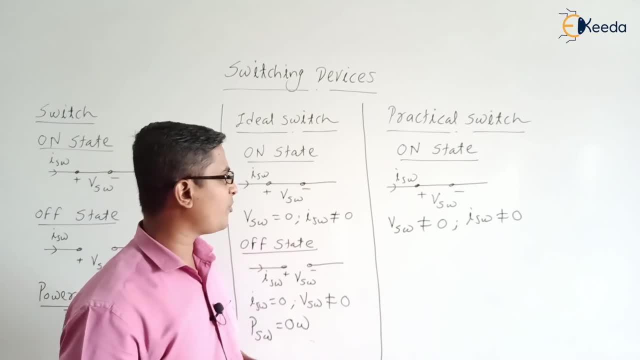 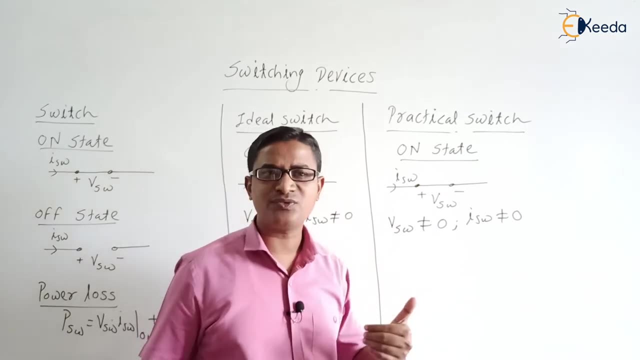 to non-zero. Is this clear to all? okay, Are you getting the point? When the practical switch is in the on state, okay, So when it is in the on state it offers some resistance. Why the practical switch is offering the resistance? Because for the manufacturing of the practical switch, we have 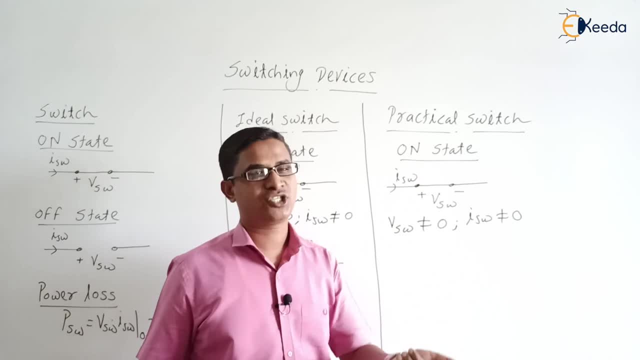 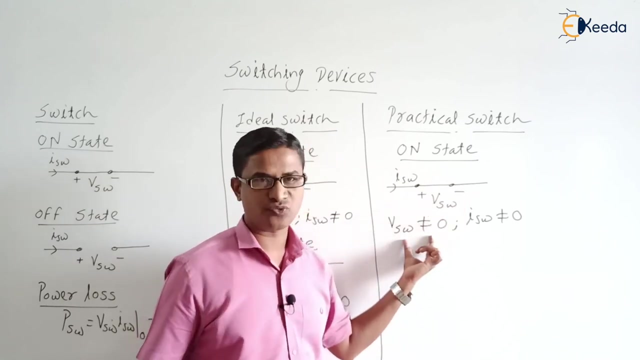 used some material and that material is having some resistivity And due to that resistivity, right This, our switch will be having some equivalent resistance. Definitely it will be a small resistance, But that small resistance is sufficient To cause some non-zero voltage drop across the switch when it is in the on state. okay Now. 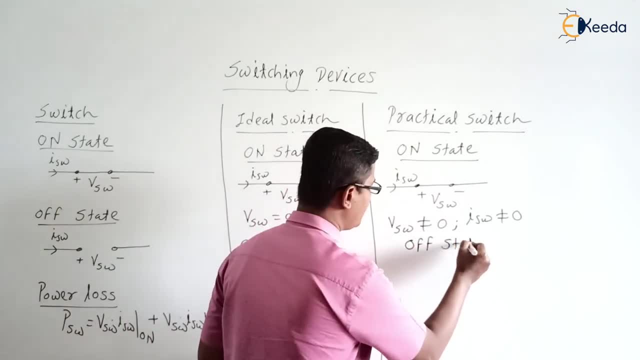 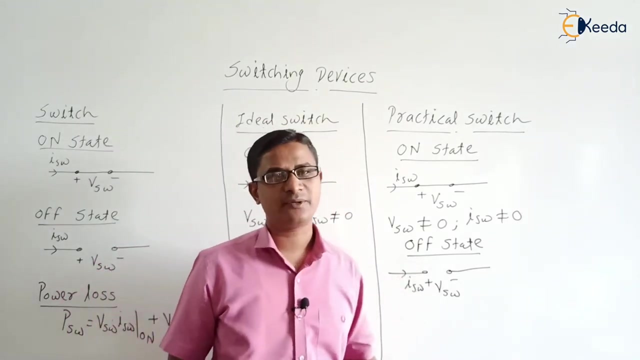 when the practical switch is in the off state. when practical switch is in the off state, okay. So here we will be having the switch. It is like an open circuit. This voltage is VSW, This current is ISW. okay, Now, when practical switch is in the off state, the current flowing. 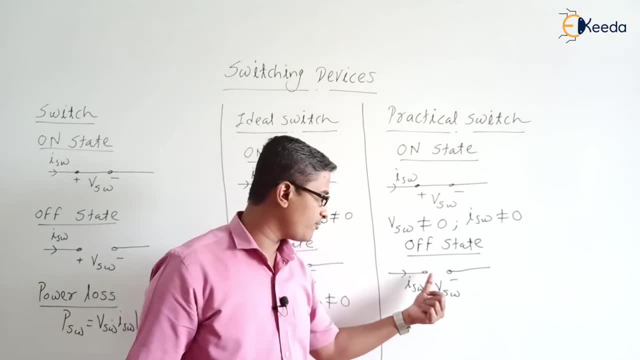 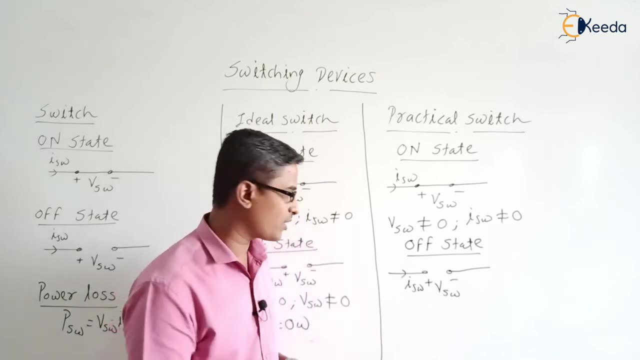 through the switch will be very, very small. Be careful. The current flowing through the switch, not a zero here. It is a small value. It is in the range of microampere. Are you getting the point, okay? So here, current flowing through the switch, that is the ISW. Yes, it is a non-zero ISW is. 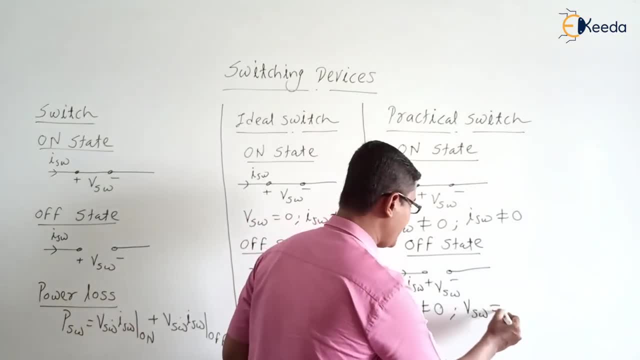 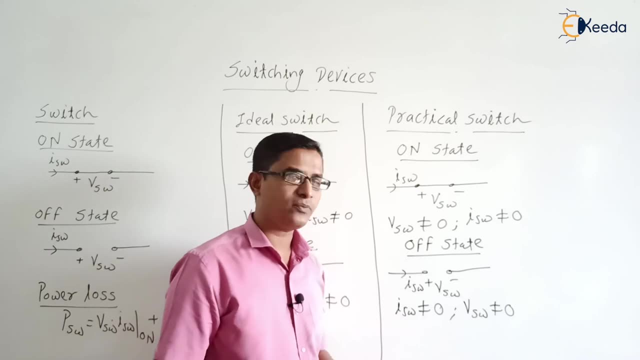 non-zero, right? And what is the VSW? Definitely, VSW is also non-zero because it is a open circuit. Because it is a open circuit, Are you getting the point Why this current is non-zero? Generally, we say it as a leakage current. Generally, we say it as a leakage current. This is a very small. 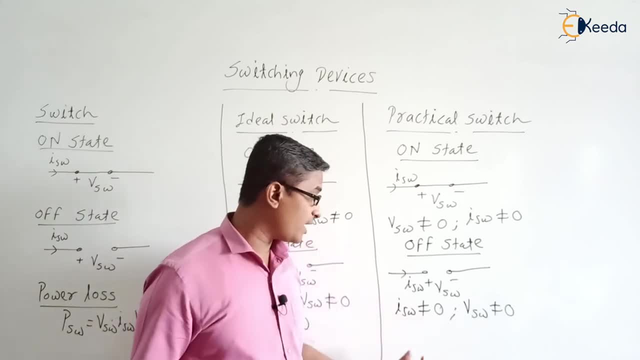 current. It is in the range of microampere. So this is a very small current. It is in the range of microampere, So microampere only okay, But it is having some non-zero magnitude, okay, And this is a VSW. 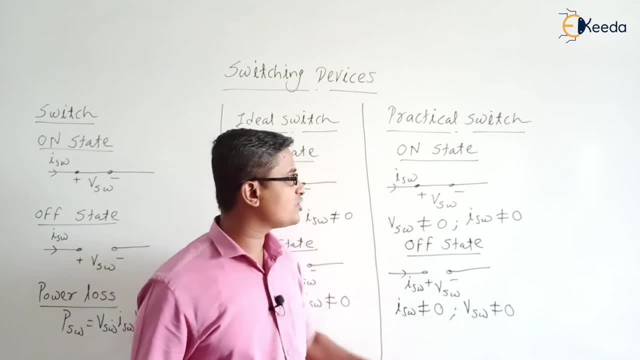 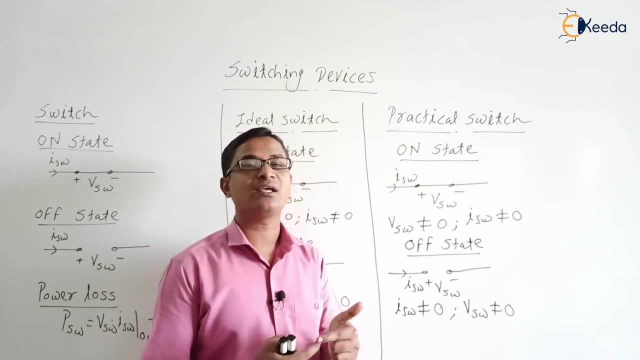 voltage across the switch. So if you check the practical switch during the on state, voltage across the switch and current flowing through the switch, both are non-zero. So what is the power loss? in the case of practical switch, when it is in the on state, It is a non-zero.